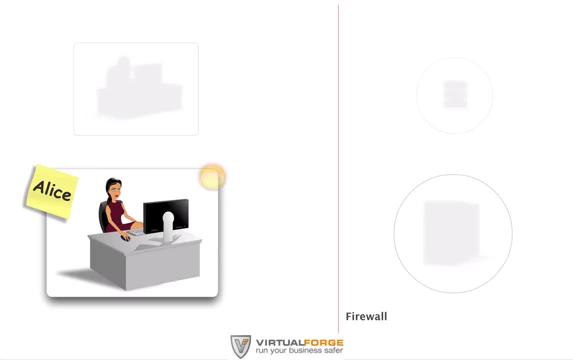 Alice, on the other hand, wants to buy a car. She will demonstrate use case 2.. Every now and then, she checks out the current cars on sale. She too, is authenticated to the application. Her identity, too, is validated by the server. 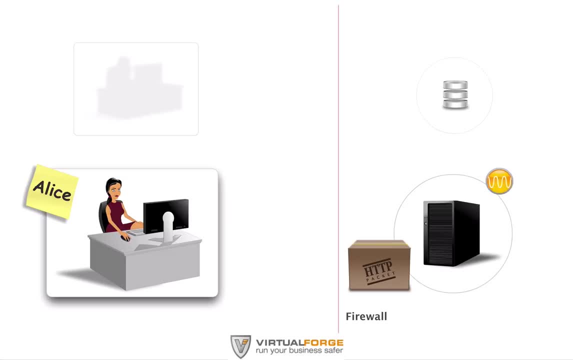 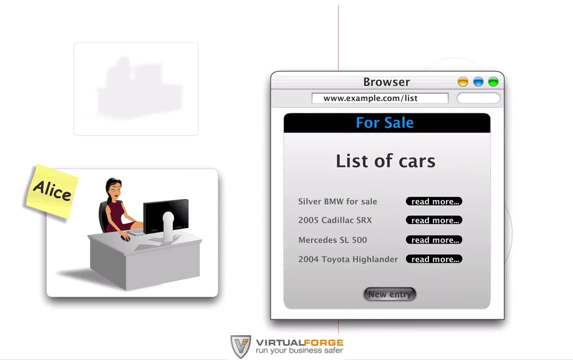 When she comes back. this time the list also includes Bob's new entry. The list of cars is rendered in her browser. Since it's new and interesting, Alice decides to have a closer look at Bob's ad. Please note that part of Bob's ad has syntax highlighting. 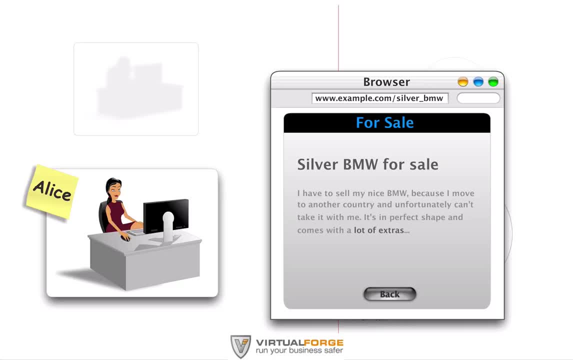 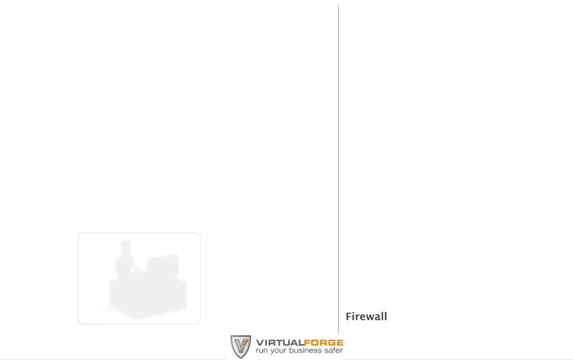 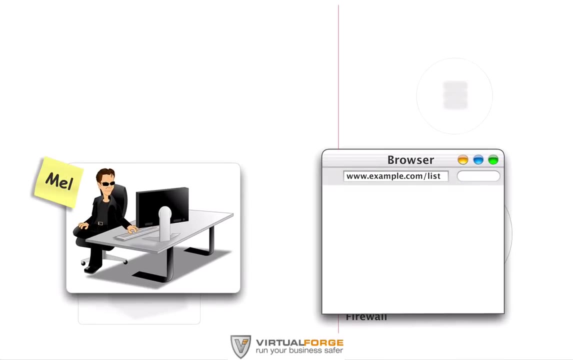 The phrase. The phrase lot of extras is bold, so that's how the application is supposed to work. Some people contribute content, others will read it. Now we need to bring in another player: Mel Mel is using his lunch break to see. 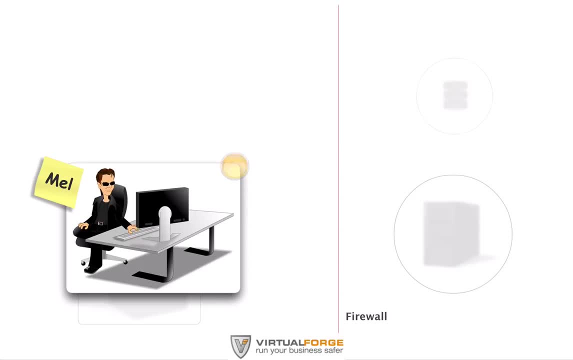 if he can hack into some systems and comes across our web server. All good hacking starts with analysis, so Mel first checks out how the application works. Basically, he does the same things Alice just did. Therefore, he receives the same information Alice just did. 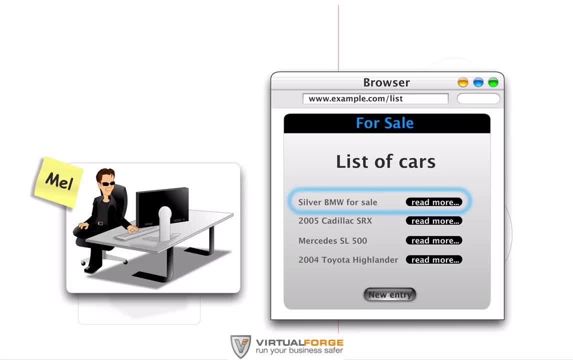 But he looks at the results a little differently. Why is there some text written in bold letters? It seems that HTML tags are allowed input, Maybe any HTML tags. Let's see if Mel can exploit that. First he needs a headline that draws attention. 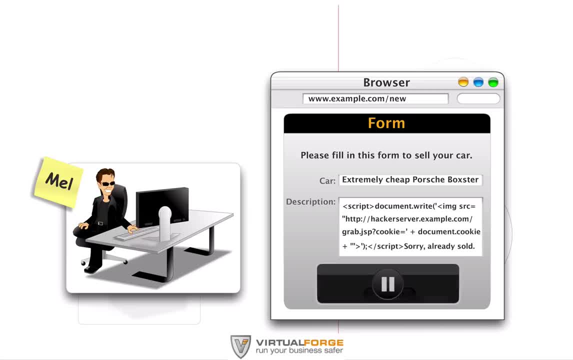 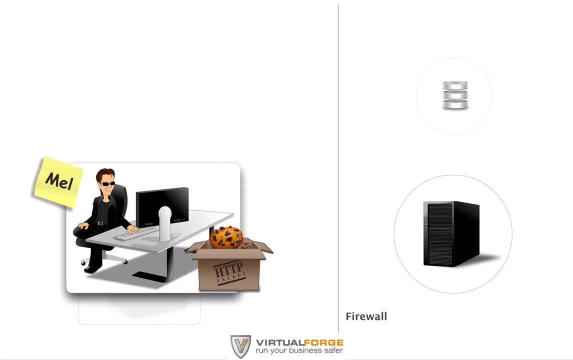 Now what if he enters JavaScript code instead of a detailed description for his car? And what if that code would read the cookie of whoever is opening that page and send it to Mel's hacker server? Mel saves his malicious ad to the server and it is processed and stored in the database the same way Bob's ad was before. 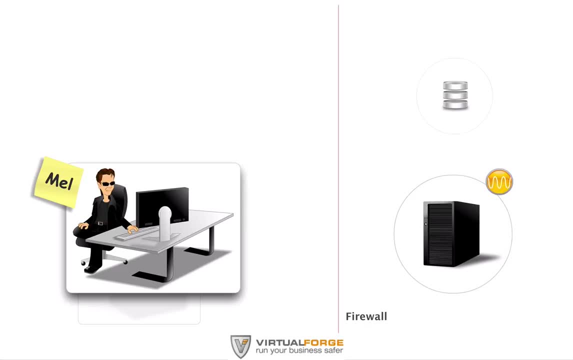 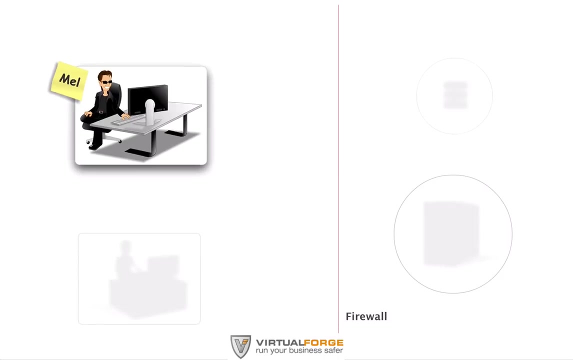 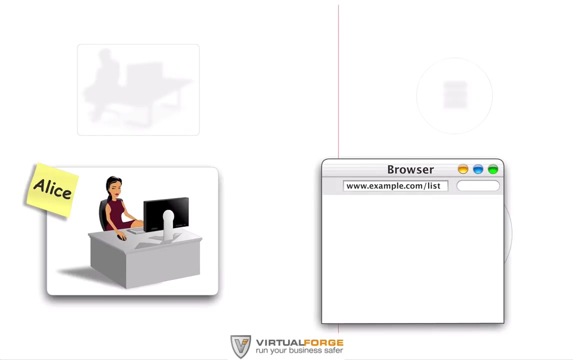 After this successful little lunch break, all Mel has to do is wait, Wait for someone else to open his malicious ad. Alice is taking another opportunity to check out if there are any new entries in the database. Again, her identity is validated by the server. 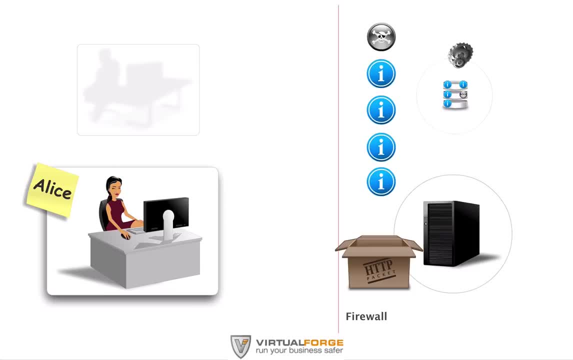 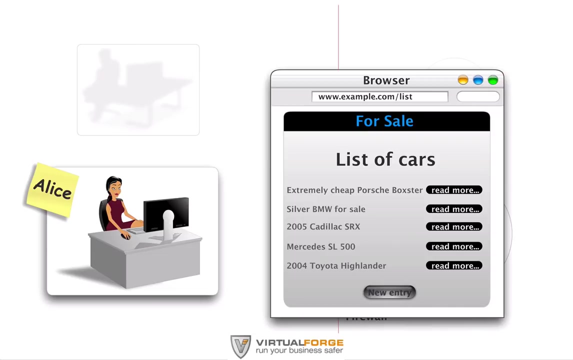 Now what if there are no new entries in the database? Unfortunately for Alice, the new list of cars now includes Mel's cross-site scripting attack. Since the attack itself is hidden in the description, it will be launched the moment Alice opens the Read More page. 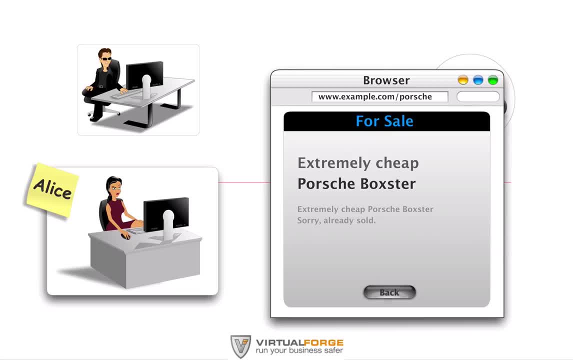 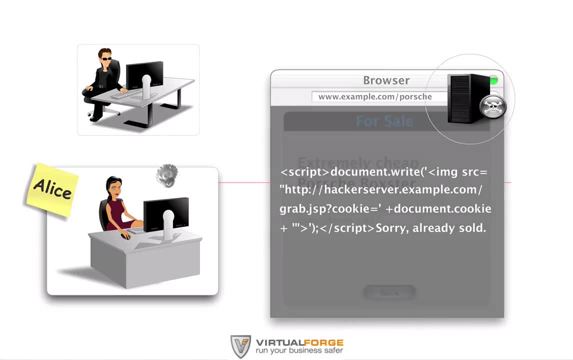 Mel's script is now executed in Alice's browser. The script is now executed in Alice's browser. The script is now executed in Alice's browser. The script is now executed in Alice's browser. It will therefore read her cookie and send it off to Mel's web server. 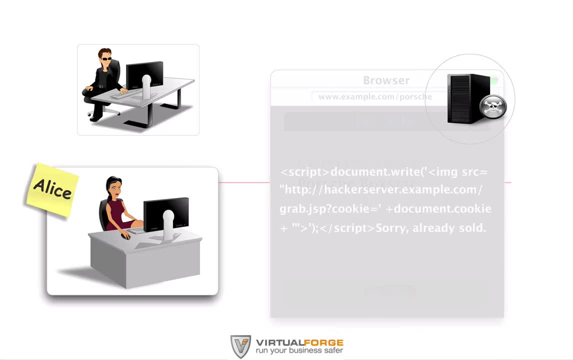 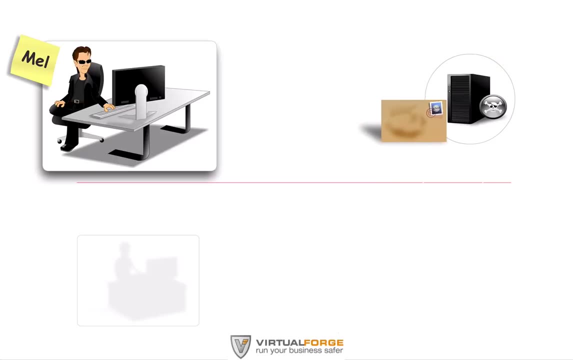